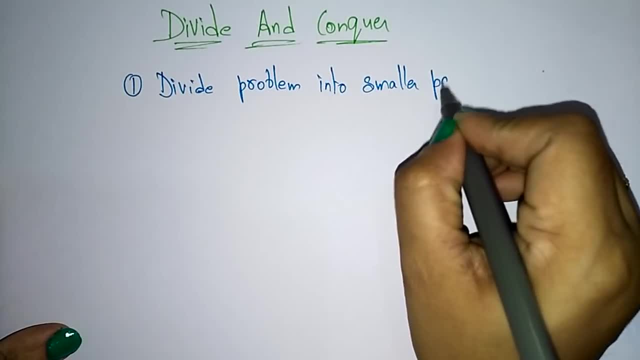 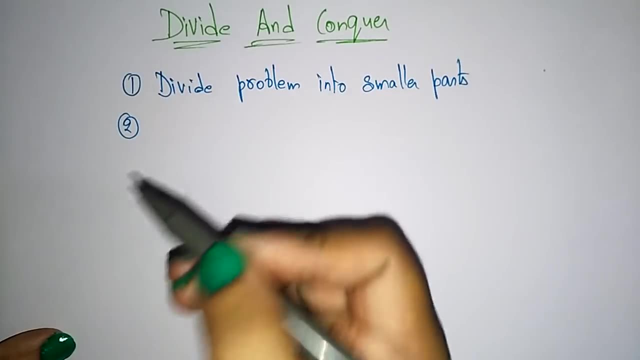 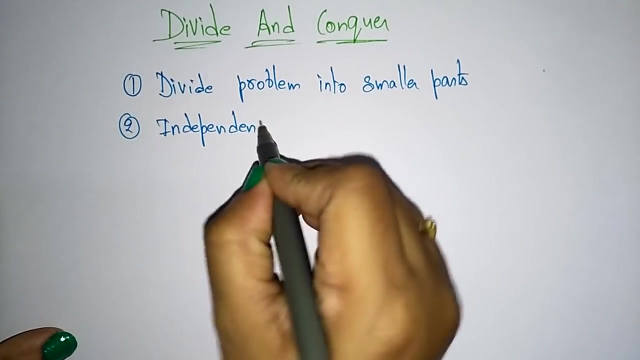 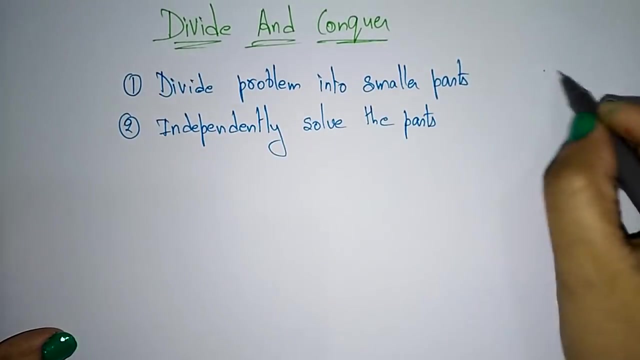 Okay, you have taken one some array and you are divided that array into smaller parts. Second, so independently solve that parts. Next you have to do: independently solve that parts. So, whatever the array you have taken, that array should be divided into two parts. 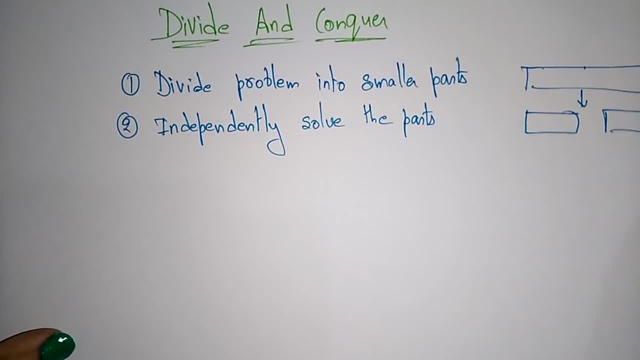 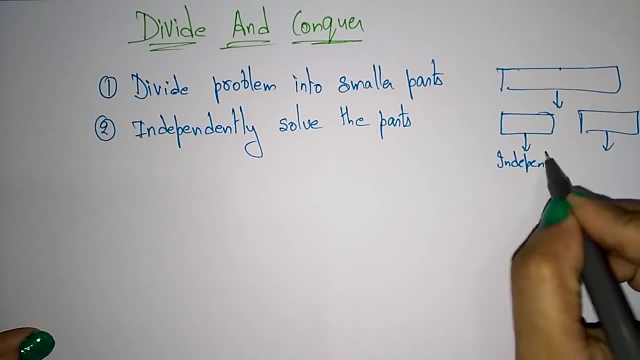 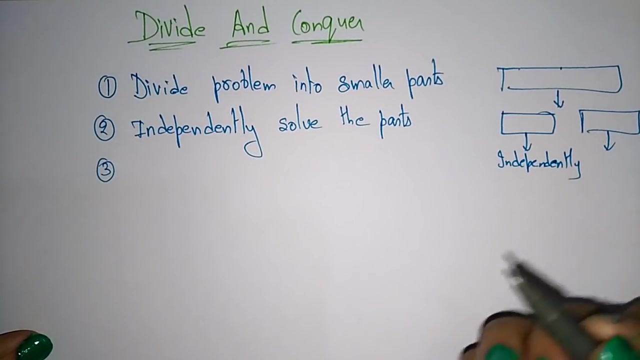 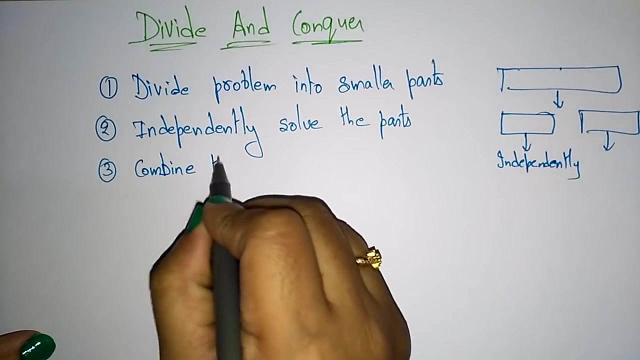 Two or more parts means divide problem into smaller, smaller parts. Again, you have to solve them independently. So you have to solve them independently. So after solving independently, you will get the solution for independent part. Then combine, Combine these solution to get independent part. 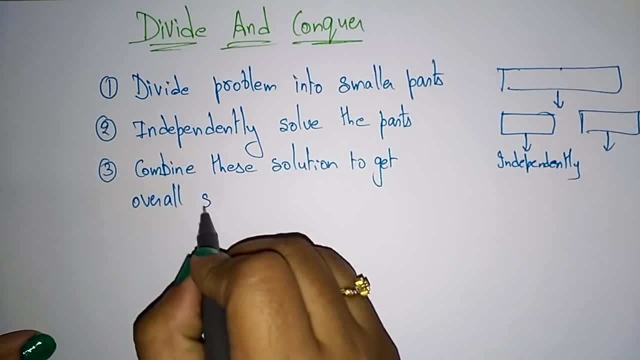 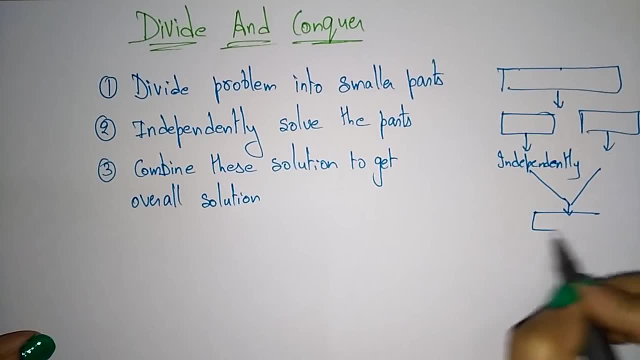 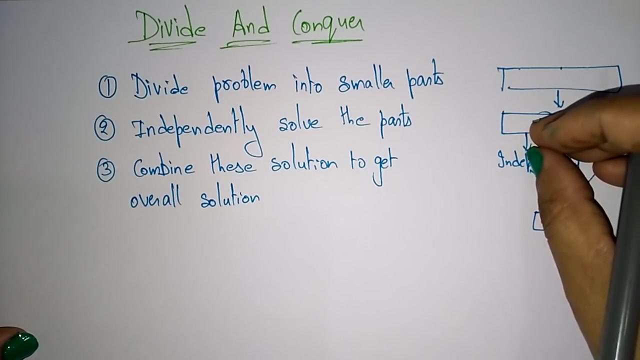 So that is the strategy you have to follow in the divide and conquer. So whenever first take problem, divide the problem into smaller parts, So all the smaller parts problem independently and combine these solution. whatever the solution you get for the independent parts, combine these solution to get the overall solution. 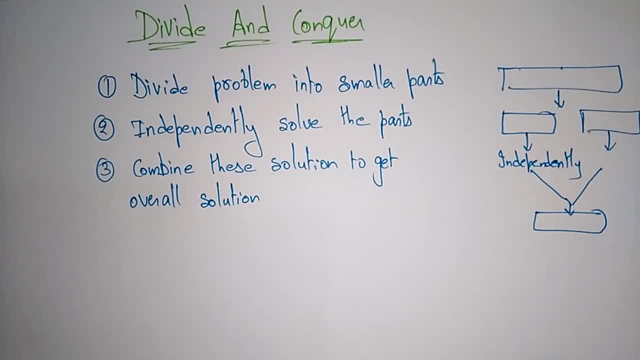 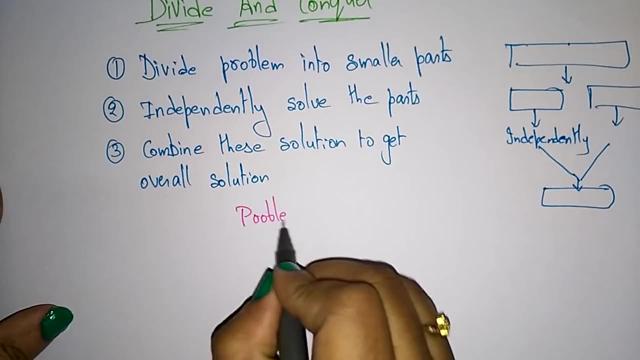 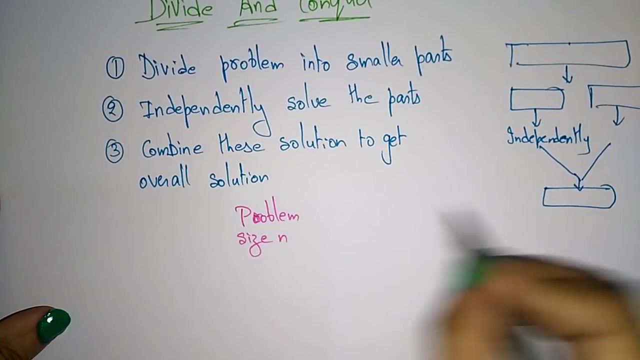 So these are the steps that are involved in the divide and conquer. So let me explain with diagrammatic. So first take the problem. So just take the problem. Let the problem. size is n Means the size of the problem is this is like n. Okay, 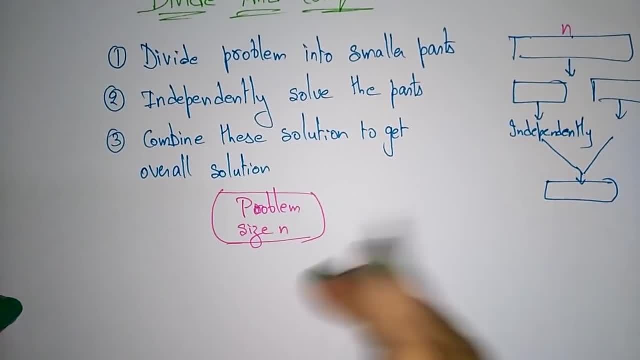 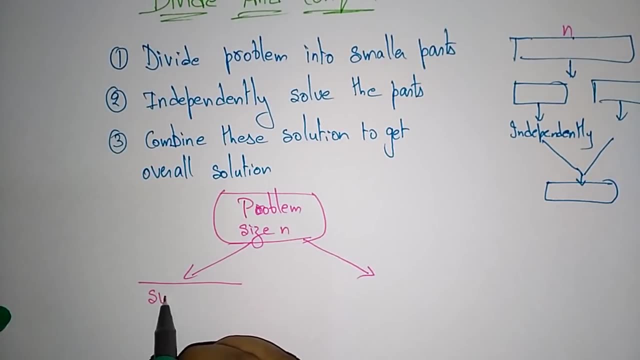 So what I have to do, I have to divide the problem into smaller problems, smaller parts. So just I am dividing into two halves. This is sub problem 1 of size. So actually the problem size is n, But I divided the problem into half So the size becomes n by 2.. 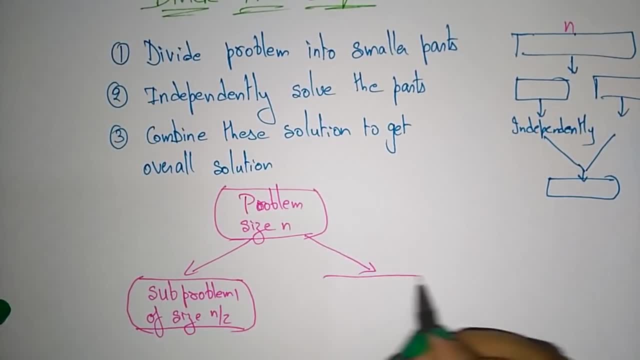 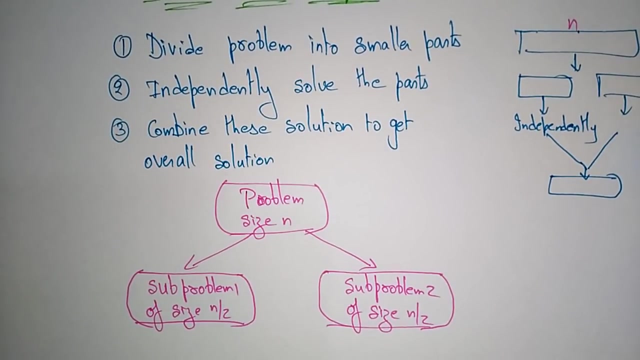 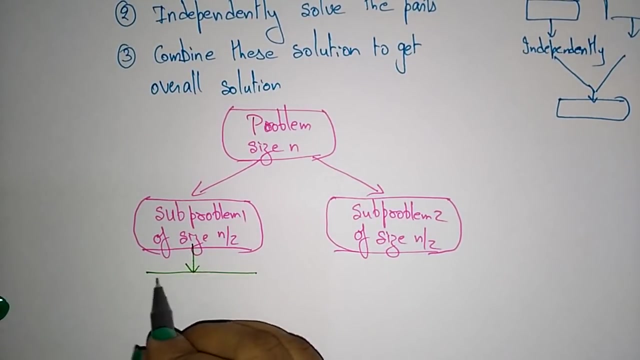 This is sub problem 1 and this is another sub problem 2, of size n by 2.. Okay, Now the problem is divided into two smaller. Now, after dividing the problem, what we have to do, We have to solve that problem. We have to solve that problem Now, solve it. After solving, you will get the solution to sub problem 1.. 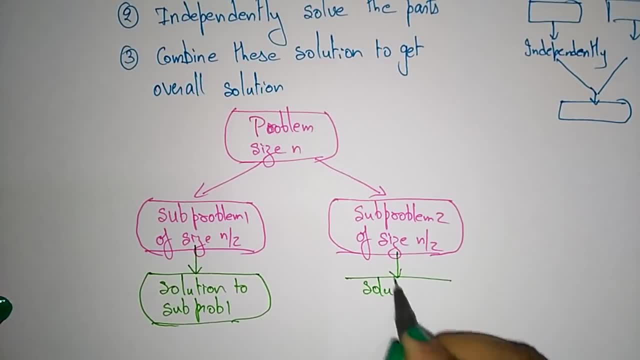 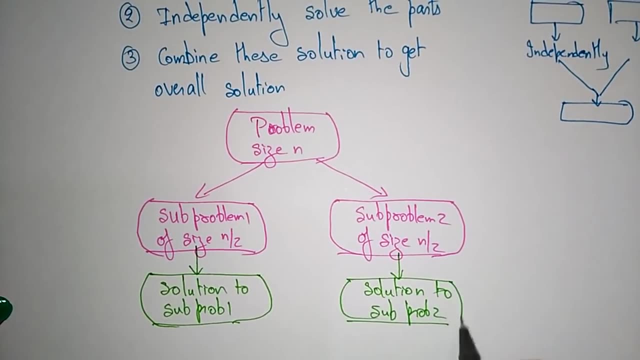 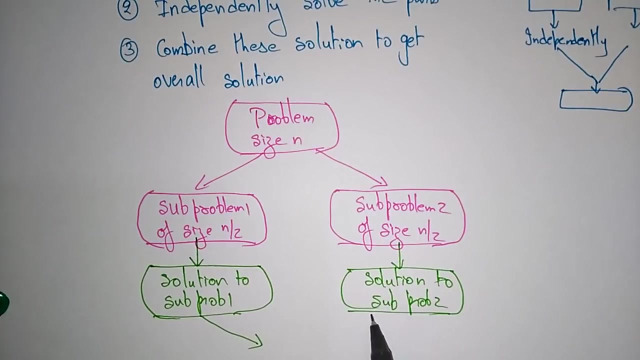 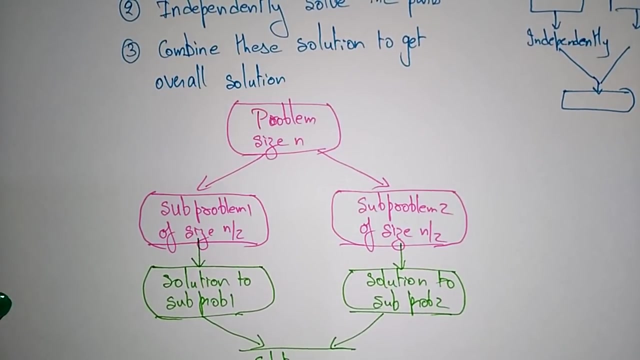 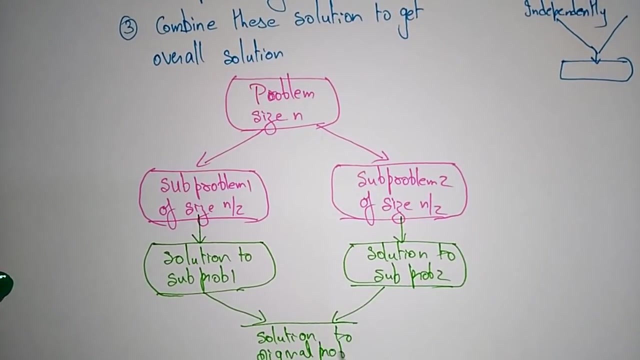 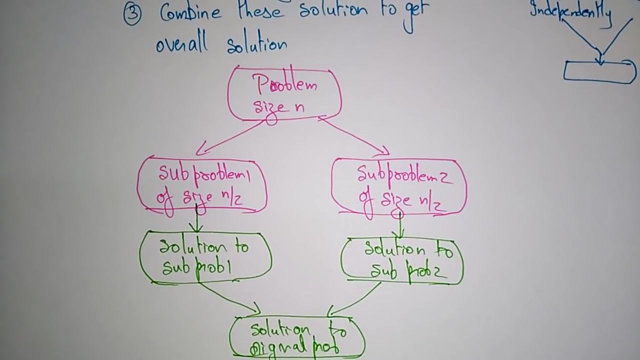 For this also. after solving, I get the solution to sub problem 2.. So I get the solutions to sub parts. Now combine all the solutions and get the overall solution. So this is the solution to original problem. Original problem. Okay, So these are the steps that are involved in the divide and conquer. 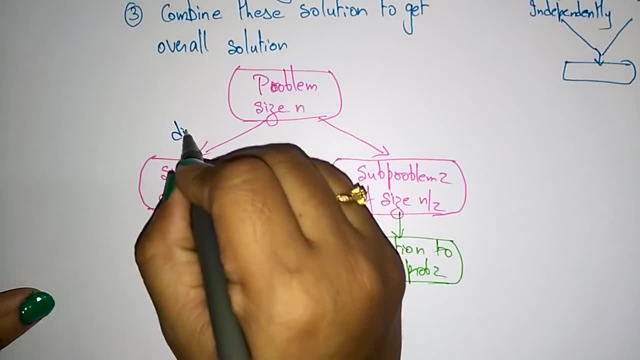 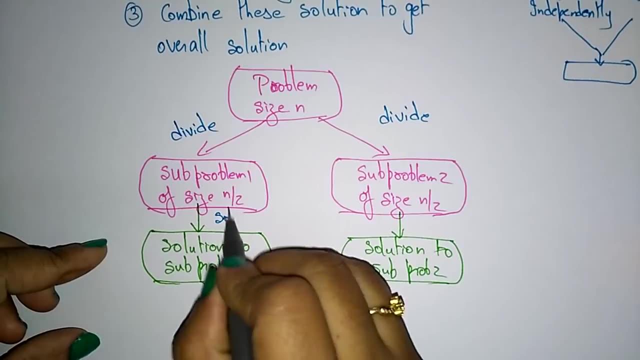 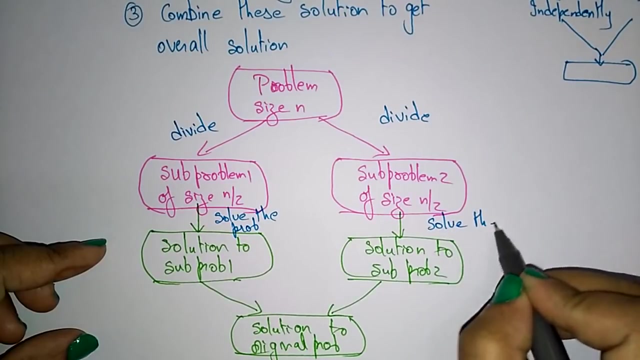 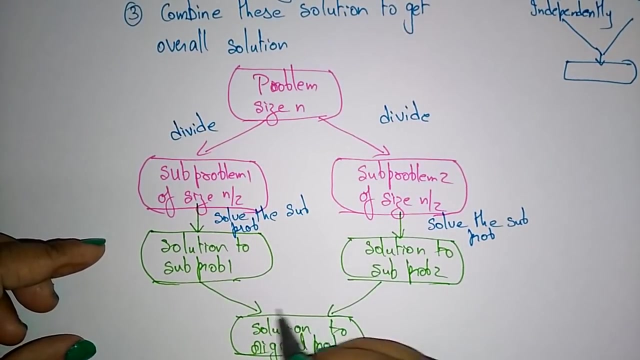 So first we have to divide the problem, Divide the problem. So after dividing, you have to solve the problem independently. Solve the problem, Solve the- you call it as a sub problem, or else Solve the sub problem. After solving the sub problem, you have to combine to get the original solution. 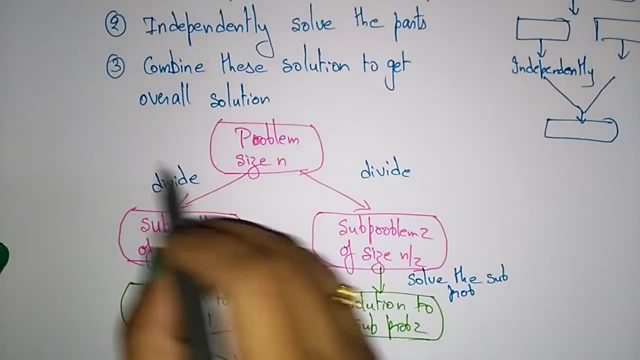 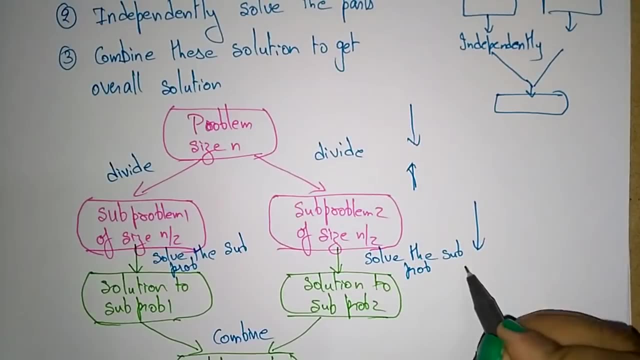 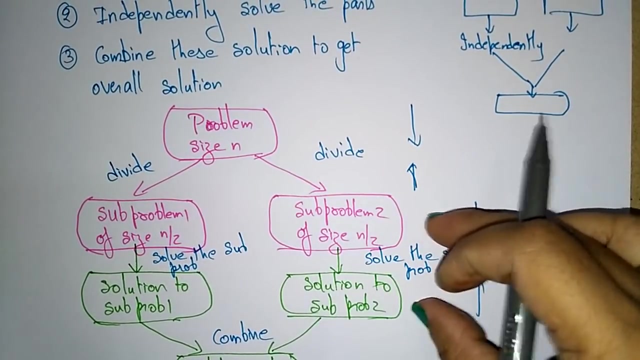 Okay, So this up to here, this stage is divide stage, This is divide stage, And this is the conquer stage. Conquer stage, You call it as this is solving the sub problem, is a conquer stage. After that, this is a combine. This is the combine stage. 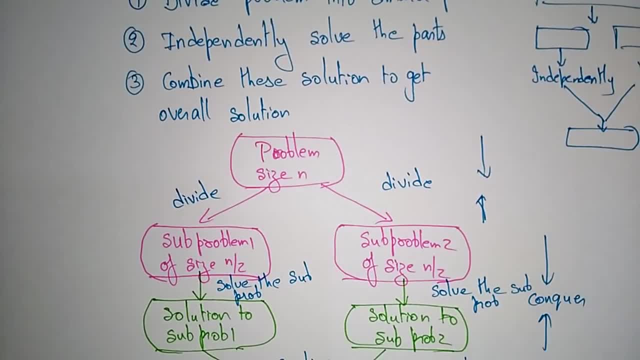 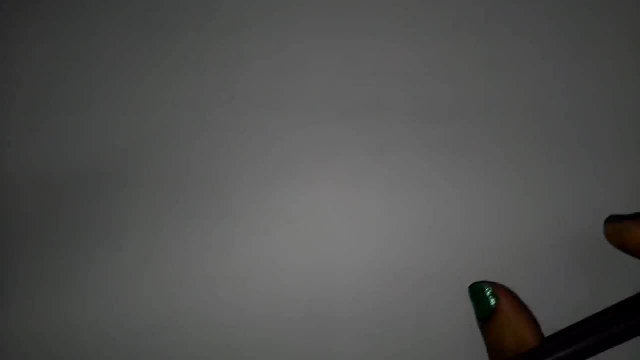 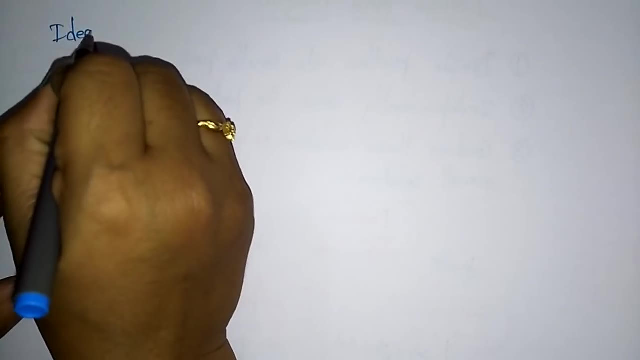 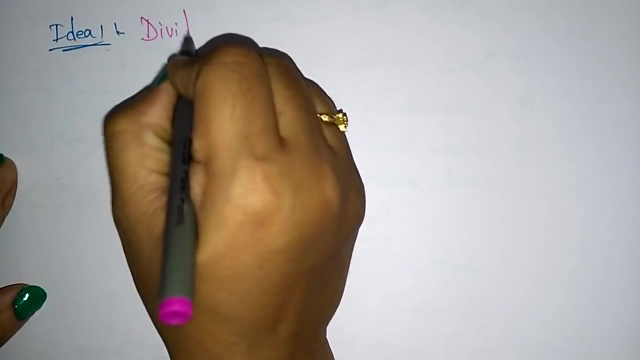 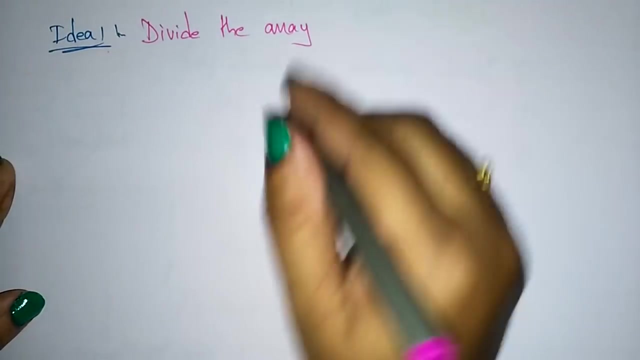 Okay, So this is the concept of the divide and conquer Conquer. Okay. So let me tell you some ideas to solve the divide and conquer problems. The first idea one, So in the idea one they are decided. we are decided that divide, the divide, the array. So whatever the problem, that is, the array you have taken into two halves. 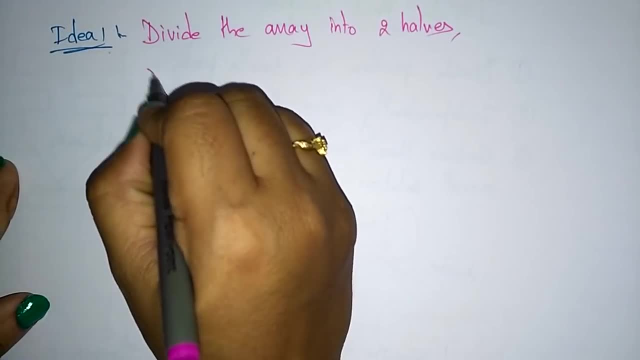 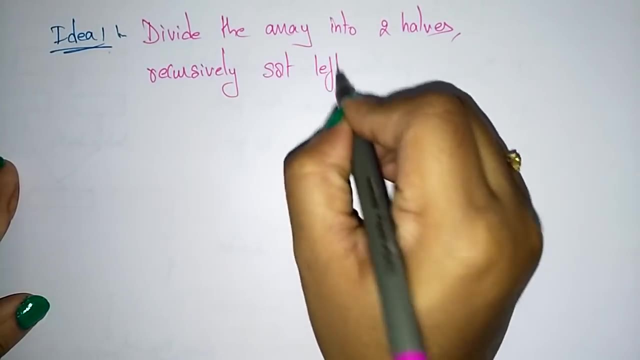 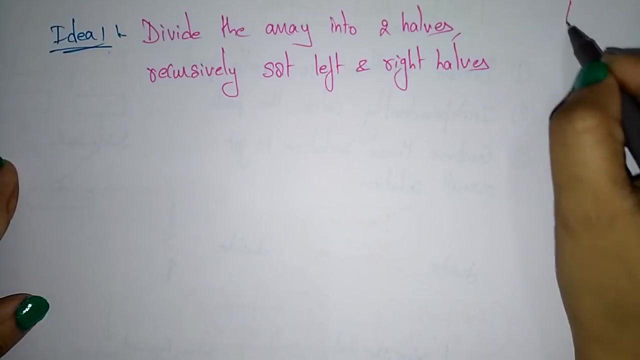 Okay, After that recursively, recursively sort left and right values, right halves. So whenever I divided the problem into two halves, okay, divide the array into two halves So one becomes the left side and another becomes the right side. So this is the left half and the right half. So first, divide the problem into two halves. 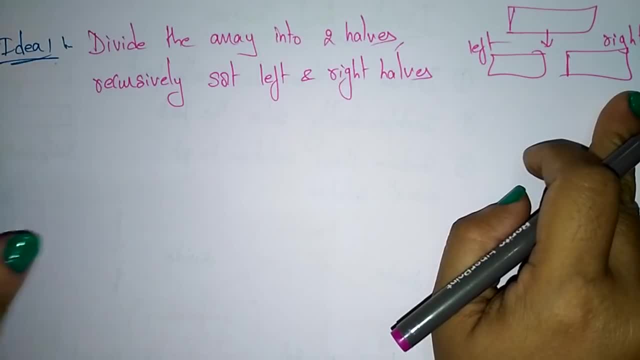 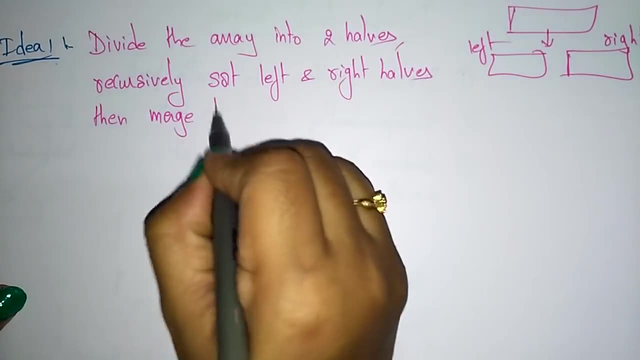 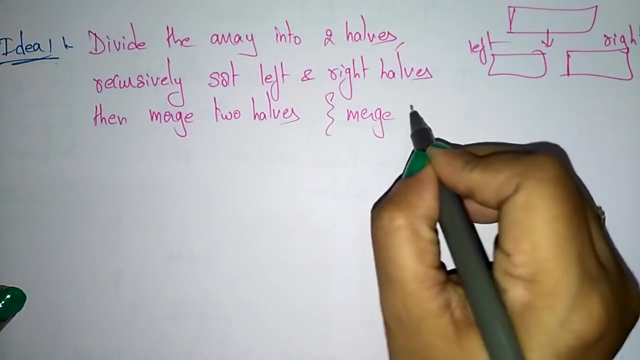 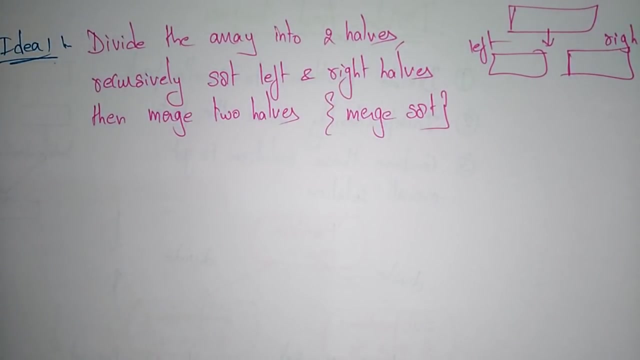 After that you have to recursively sort the left and right halves. So after recursively sorting then merge two halves. So this you call it as a merge sort. So this is the technique of merge sort. So the merge sort will divide the array into two halves and recursively sort the left half and the right half. Again it combines two and merge the two halves. 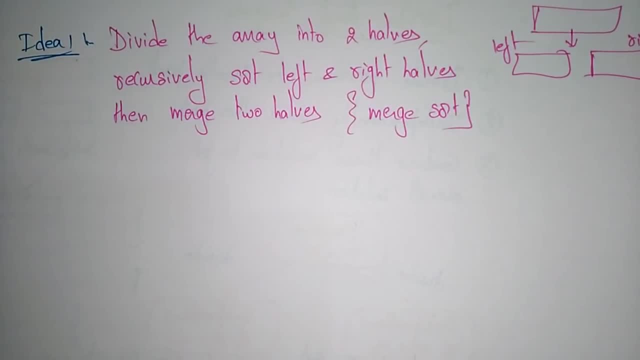 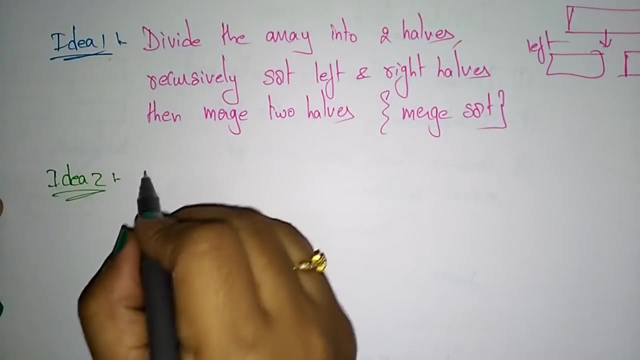 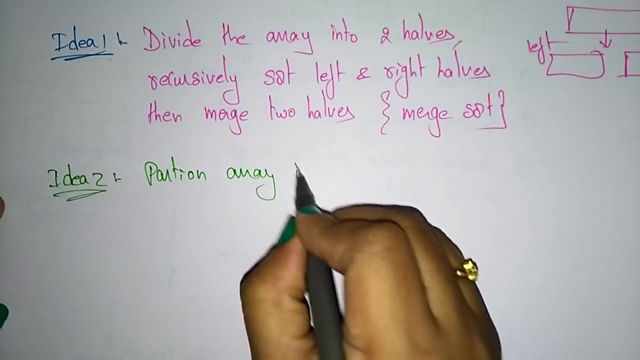 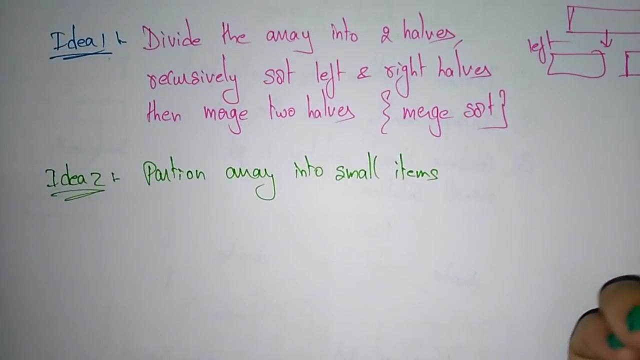